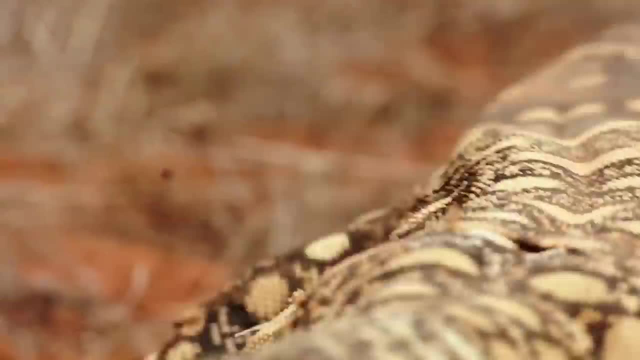 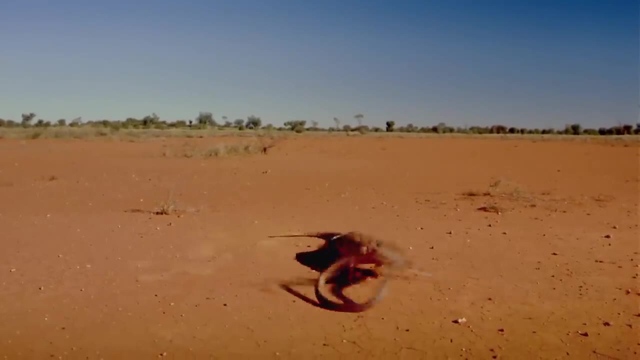 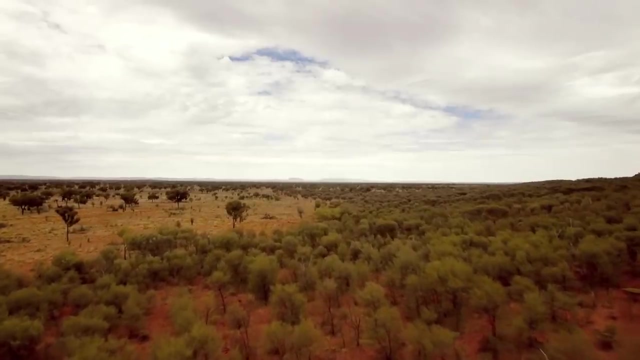 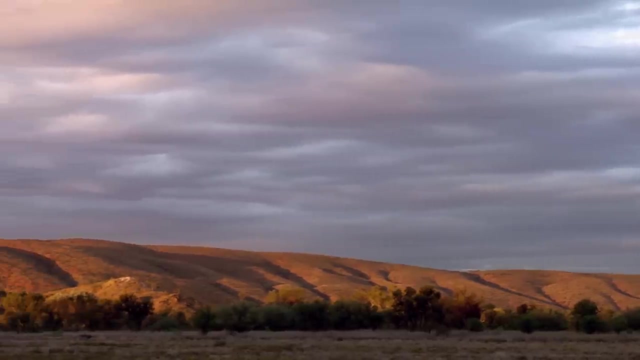 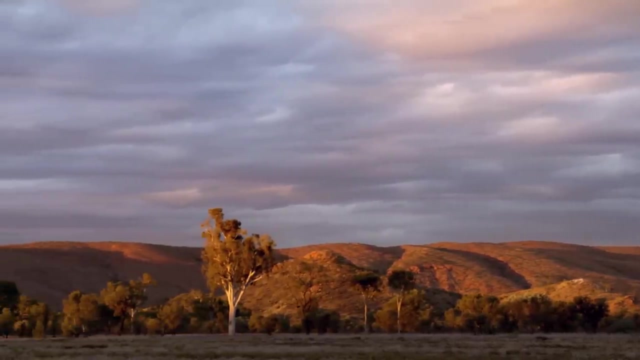 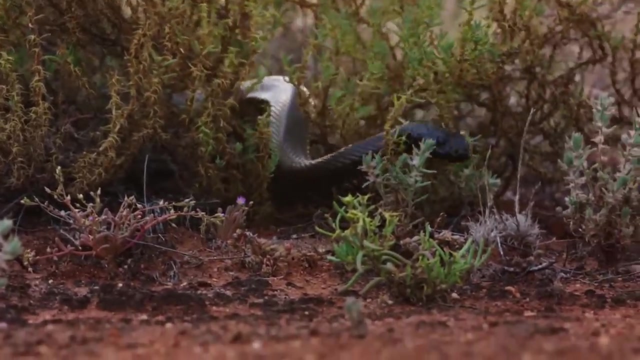 helps subdue its prey. The Perenti isn't the only venomous reptile in the Australian desert, and it certainly isn't the most dangerous. Australia is home to the 10 most venomous snakes in the world. This snake has just shed its skin. 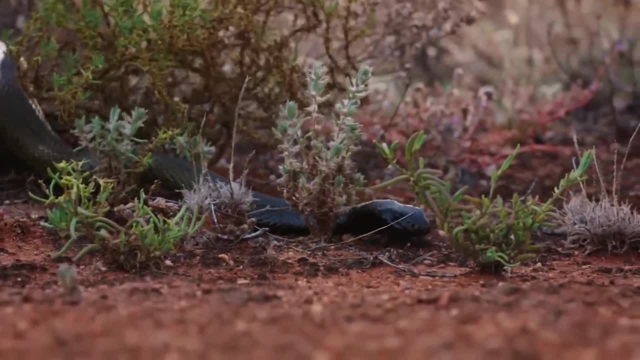 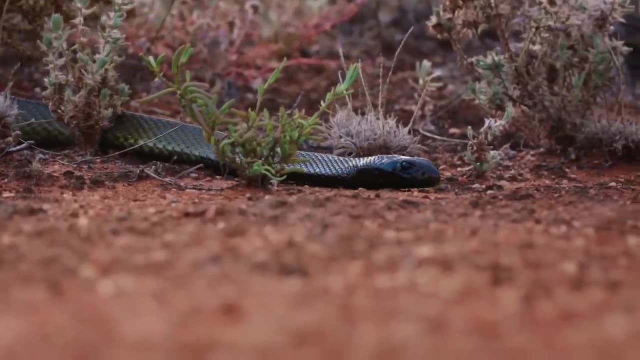 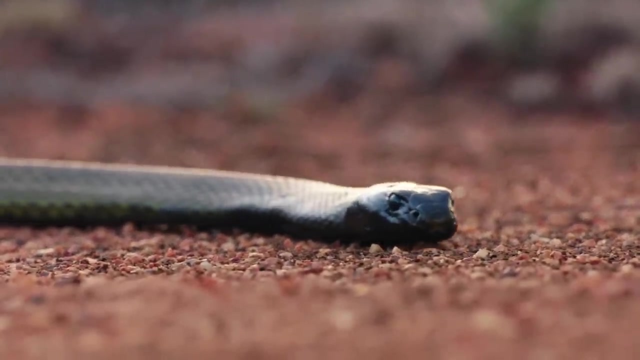 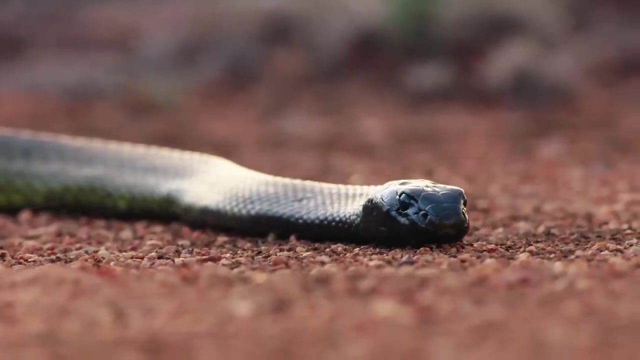 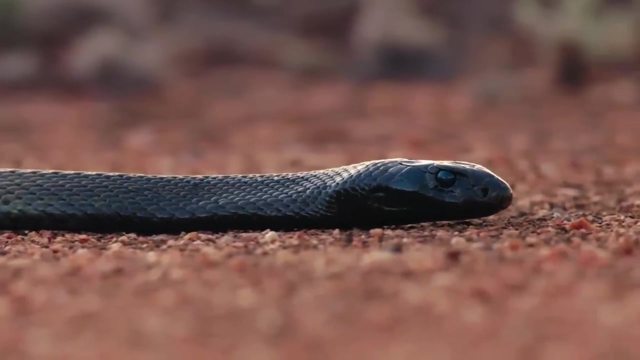 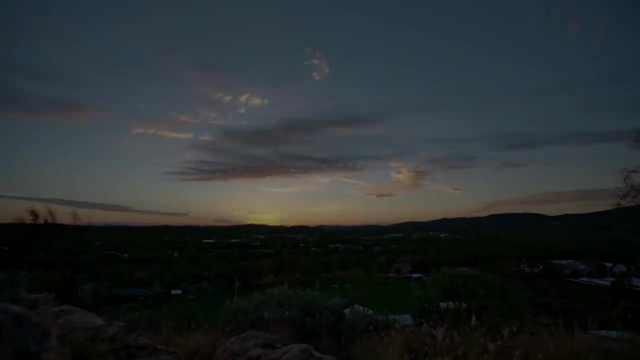 It's at its most beautiful. It's also the most venomous snake on earth: the inland taipan. It's estimated that one bite delivers enough venom to kill at least 100 fully grown humans. Desert snakes look for dark, cool places. 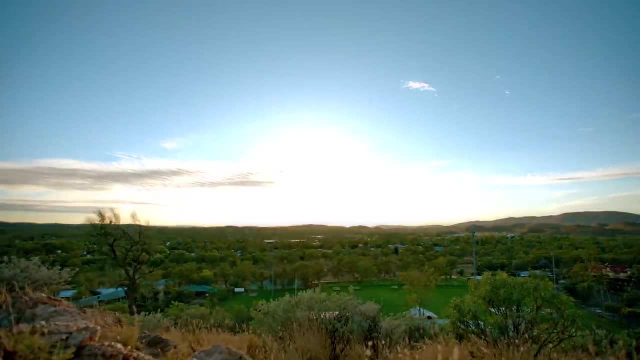 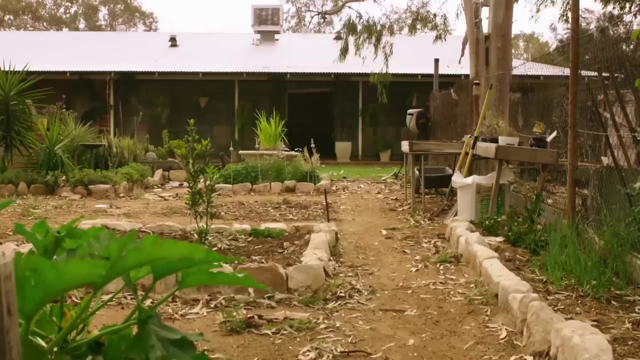 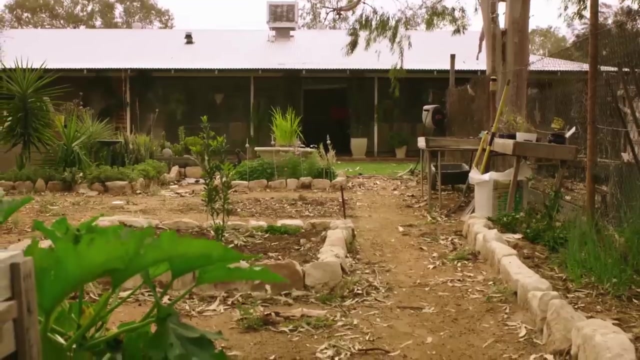 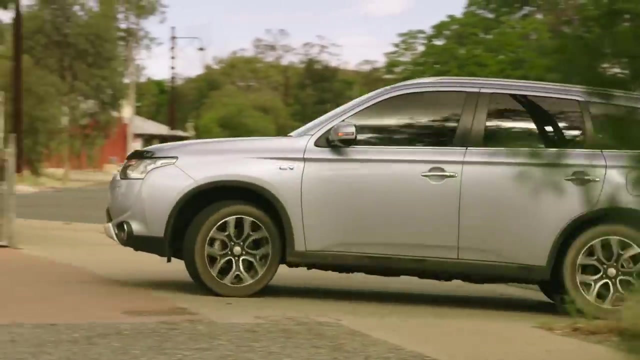 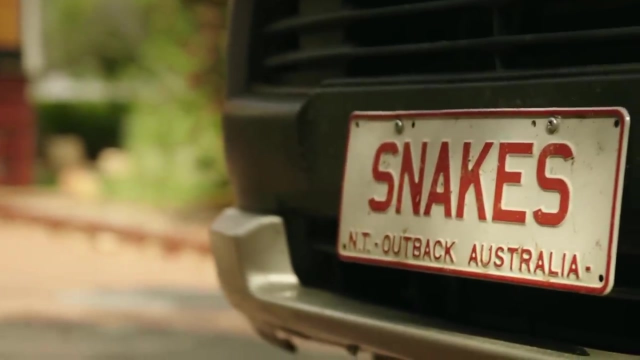 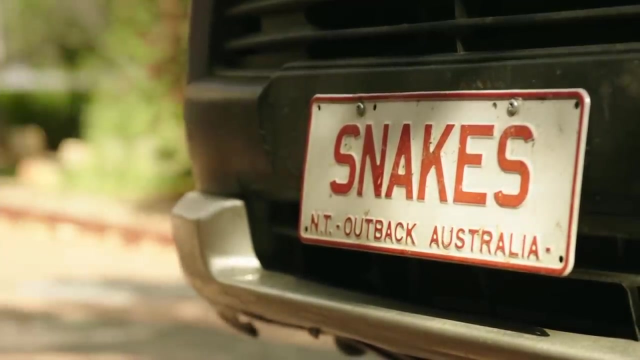 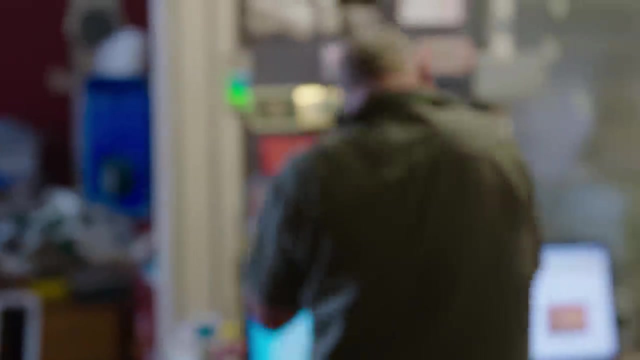 to escape the sun. Sheds and even houses make good sheltering spots. The snake removal team in the town of Alice Springs are on standby 24 hours a day, seven days a week. Rex and his staff deal with up to four call-outs a day to remove deadly snakes from local homes. 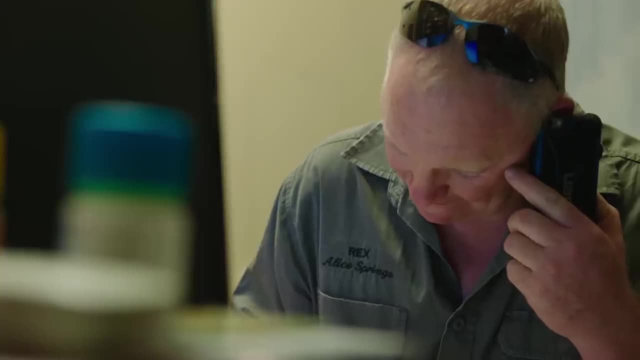 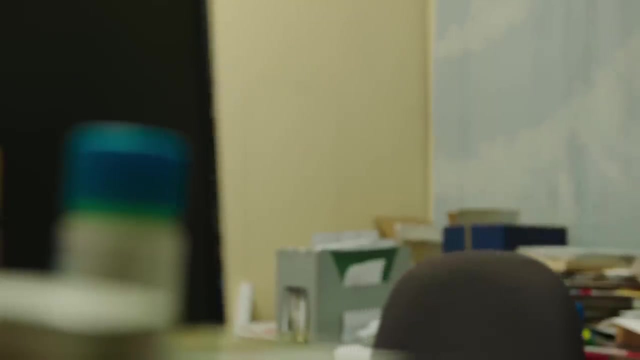 OK, what's your address? Oh yeah, are you still watching it? Yeah, no worries, OK, I'll be there shortly, See ya. Every call-out is treated as an emergency. Look like that's it. 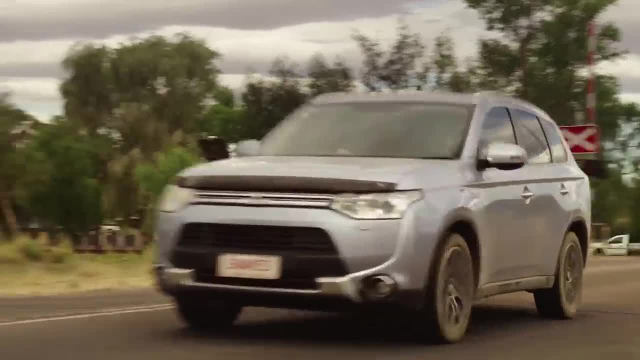 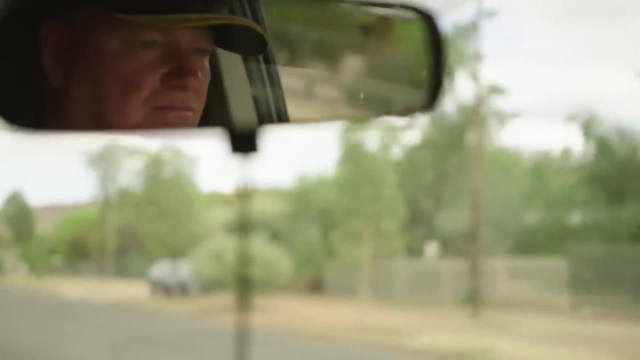 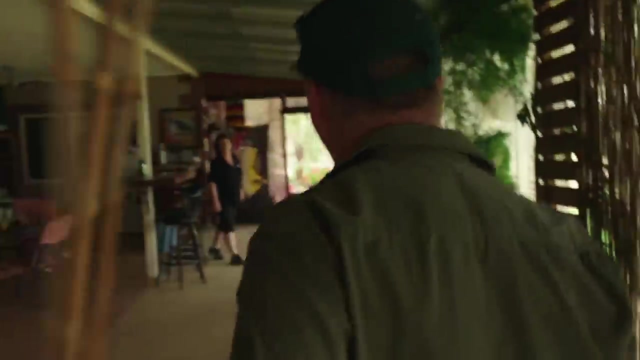 Absolutely wanted to take it. The 맛있ies are coming right now. Wow, If there's a venomous snake in a house, it's potentially life-threatening. Oh how you going, Rick. Good, What have you got for me? 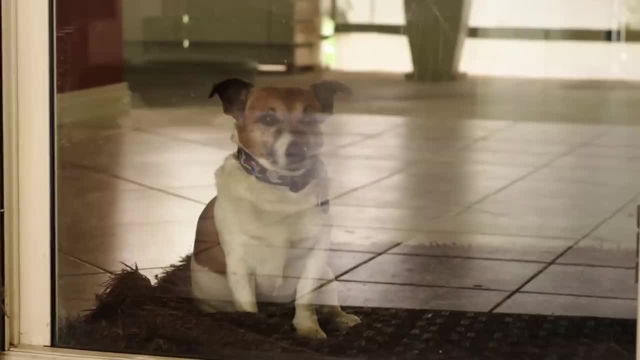 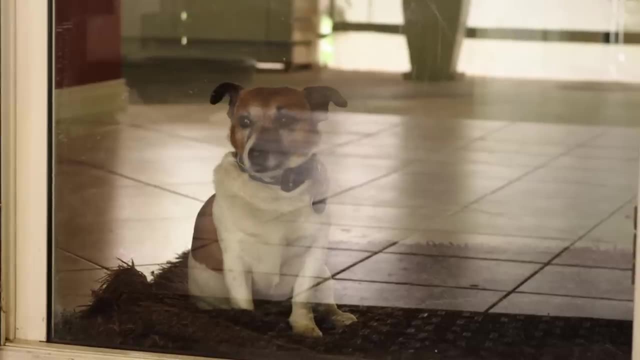 Iglong steak? Probably another western. He was a goldy brown colour. Toby the dog has been locked away. His mother was killed by a western brown snake. I'm just going to clear this out the way first, Cathy, So when you're dealing with snakes you've got to have enough elbow room just to get. 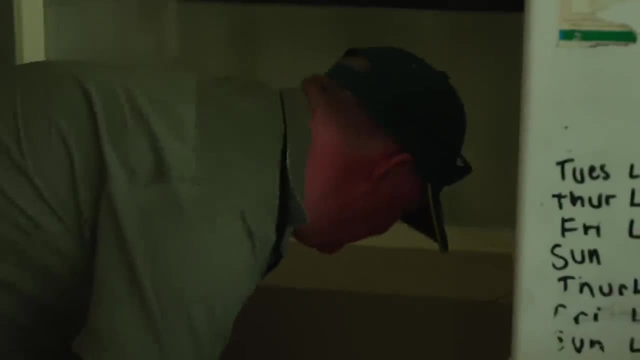 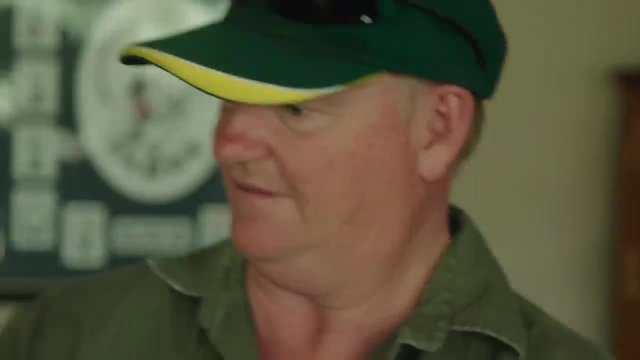 in there and manoeuvre with them. Just make that a block there so he can't go past there And here you go. Cathy, Can you get rid of that for me somewhere? Yeah, Oh yeah, Is he there? He's there, Cathy. 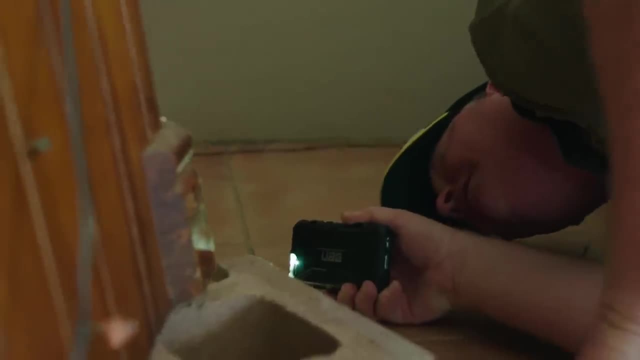 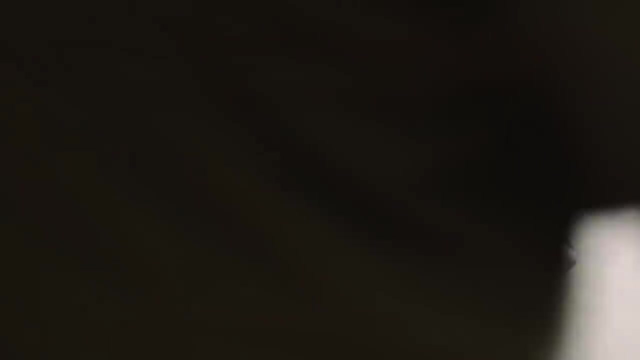 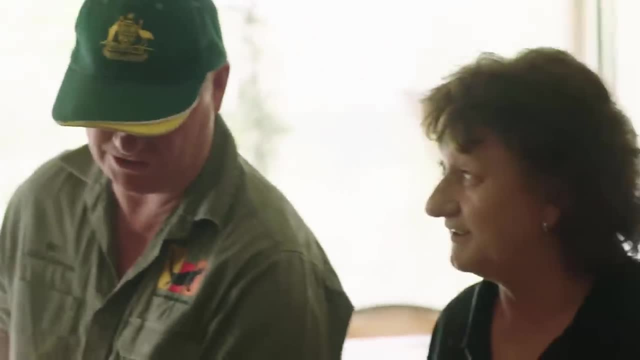 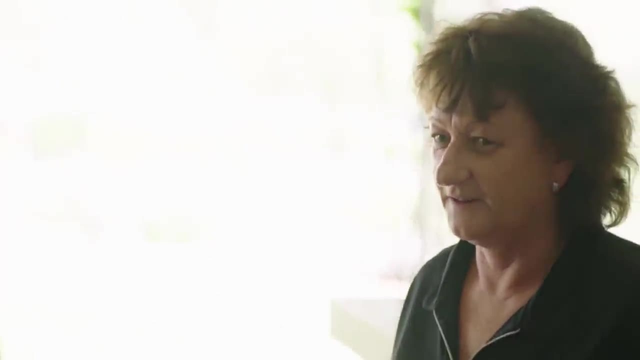 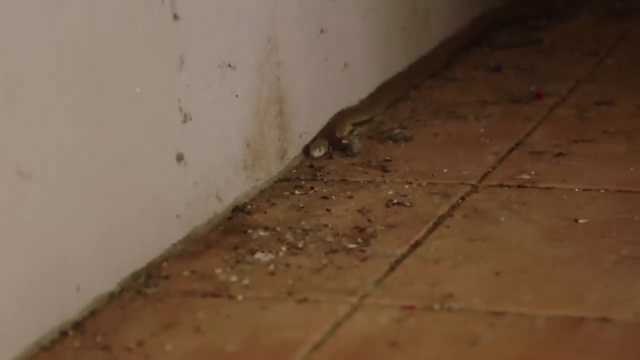 So, Cathy, if you just stand back here and if you can watch for me that side there and that side there, just to make sure he doesn't come out the back, Okay, He's coming this way. The Australian brown snake, the second most venomous snake in the world. 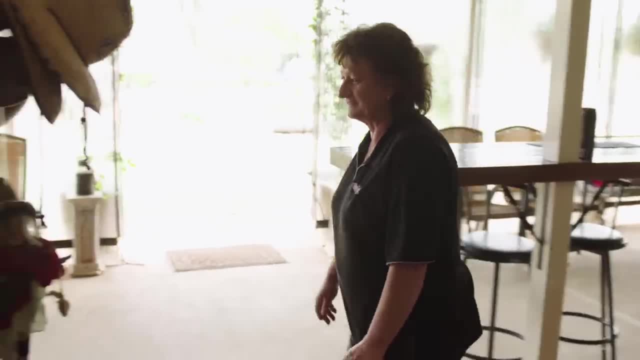 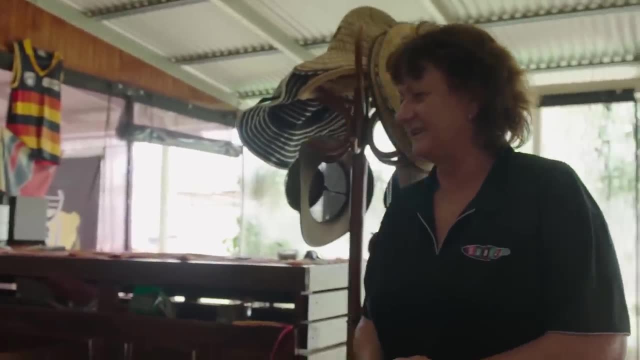 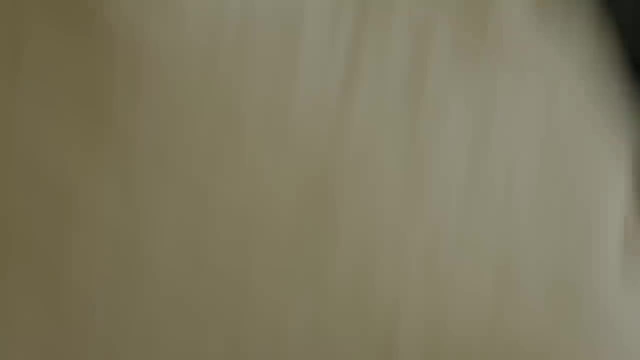 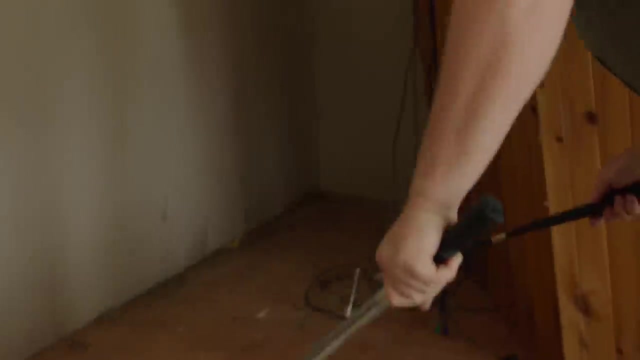 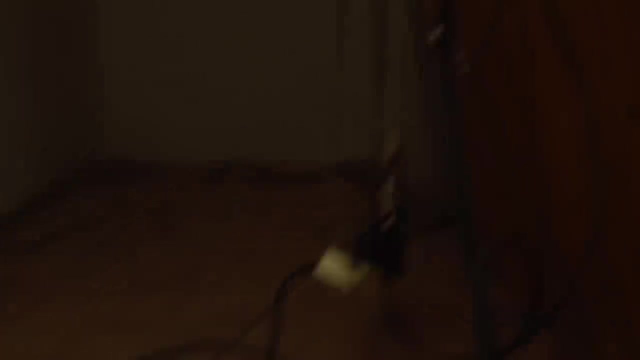 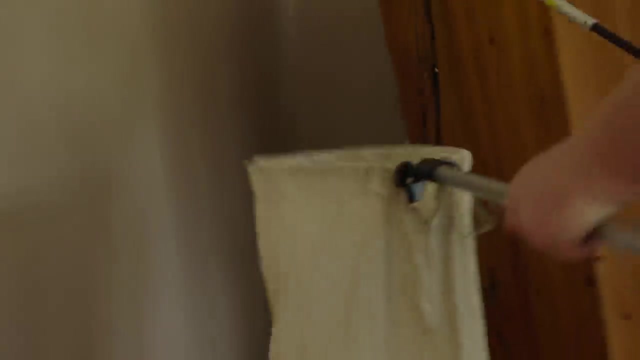 Get him. Oh, he's going around the back. Hang on. Fast and aggressive when disturbed, the Australian Western Brown Snake is notoriously dangerous to capture. Alright, all done, Cathy, I'll just bag him up for you. There you go. 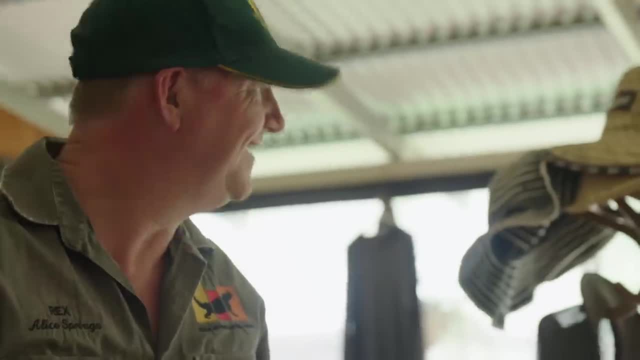 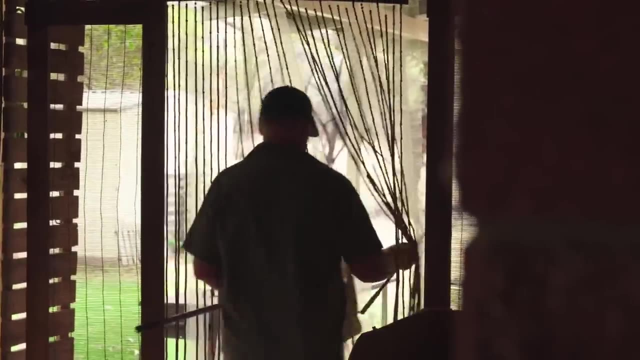 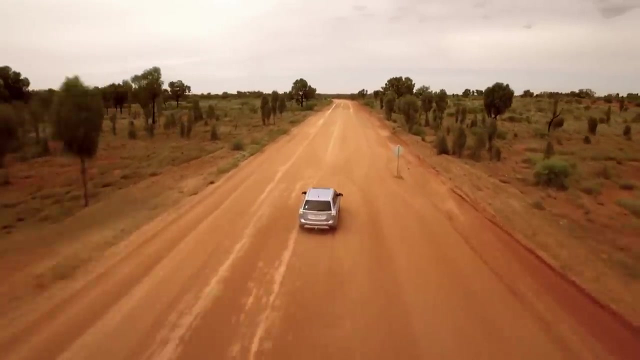 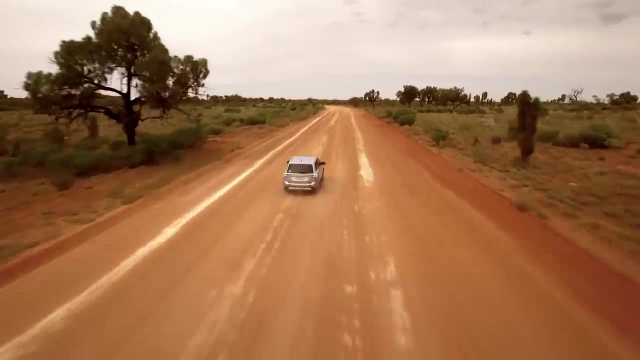 All done. He wasn't too bad, really, Safe and sound. Yeah, yeah, we'll take him out, bush, and go and release him for you. Alright, thanks for coming. Thanks, Cathy Rex is on his way to a property where the snake will be safe and well away from houses.